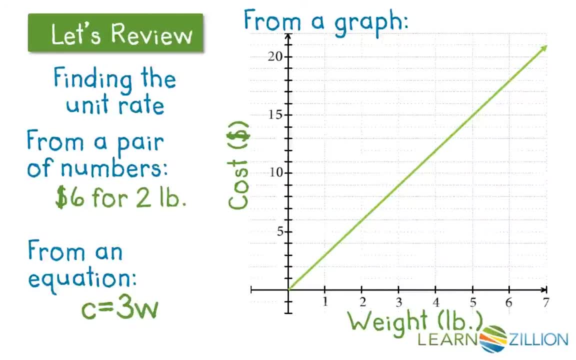 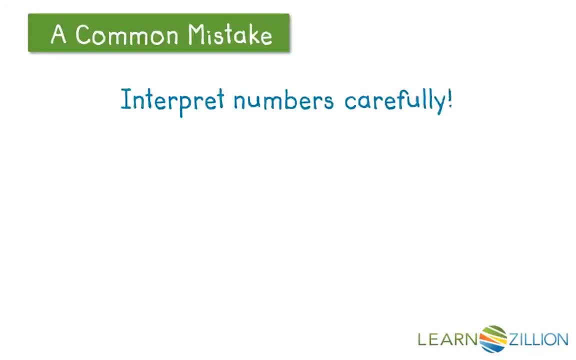 In this case, 1 pound corresponds to $3.00, so the unit rate is $3.00 per pound. When answering the type of question that we're going to answer in this lesson, we need to interpret numbers carefully. For example, which of these two stores offers the better buy? 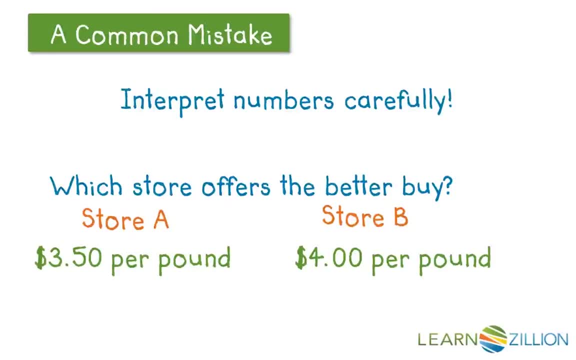 We can tell that $3.50 is less than $4.00.. Do we want fewer dollars per pound or do we want more dollars per pound? In this case, better buy means fewer dollars per pound, But we've got to be careful not to automatically pick the larger number or the smaller number without thinking the situation through. 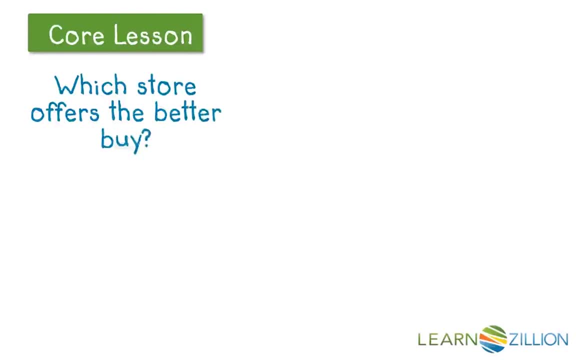 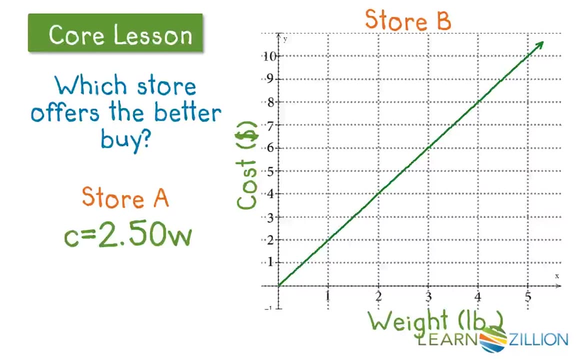 Okay. So which of these two stores offers the better buy? Store A's pricing is represented by this equation and Store B by this graph. Let's figure it out by comparing the unit rates. The unit rate for Store A is $2.50.. 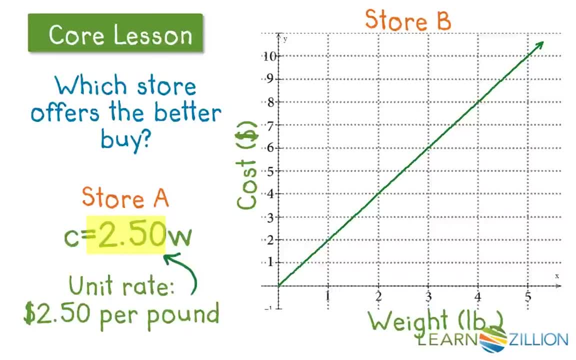 $2.50 per pound. Store B has a graph. We can find the unit rate by finding 1 on the x-axis. We see that 1 pound costs $2.00, so the unit rate is $2.00 per pound. 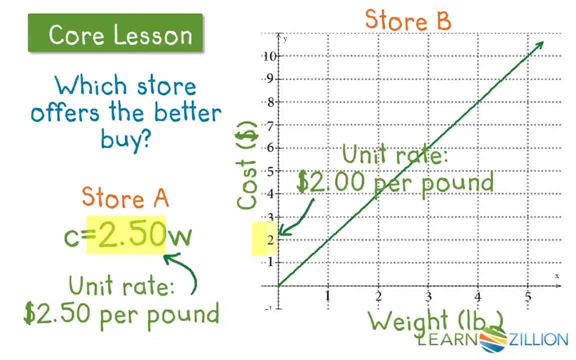 Since we're talking about which is the better buy, the answer is going to be the store that offers that costs fewer dollars per pound. So Store B is the better buy, because $2.00 is less than $2.50.. By the way, this is what the graph of Store A's pricing would look like. 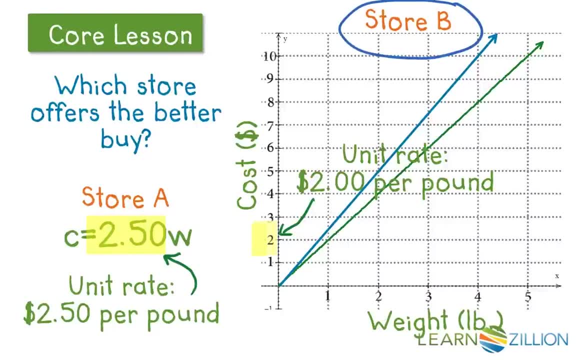 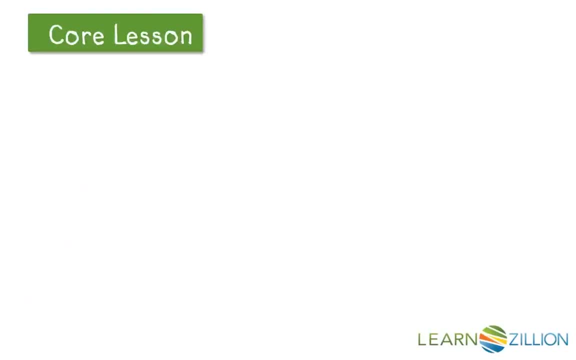 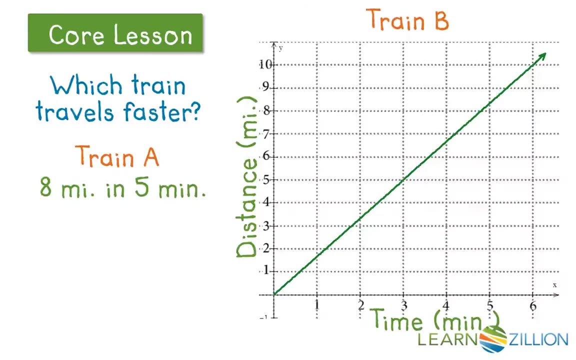 Notice that it's steeper than Store B's graph. That's because you're paying more dollars at Store A for every pound. Which of these trains is traveling faster? Train A travels 8 miles in 5 minutes, and Train B's distance and time are shown on this graph.